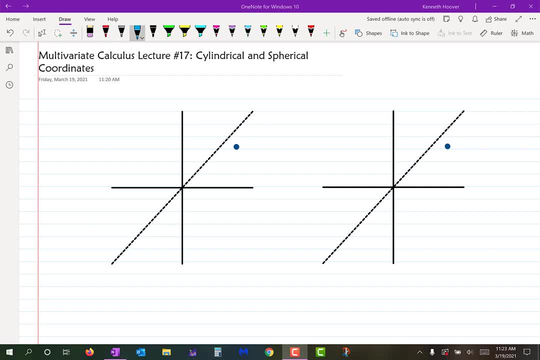 Okay, today we're going to talk about cylindrical coordinates and spherical coordinates, So let's start by just looking at how to plot a point in rectangular coordinates. Okay, so you already know how to do this. What we do is we measure how far along the x-axis do we need to go to get next to the point. 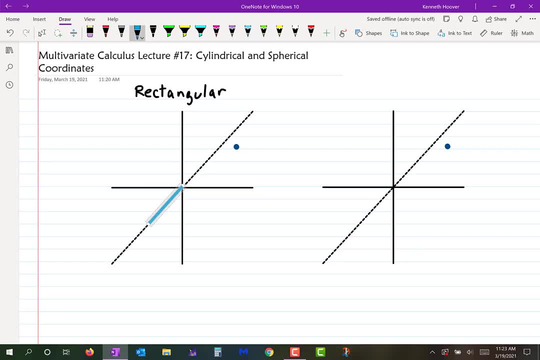 Okay, and then that is our x coordinate. And then we go perpendicular to that, Parallel to the y-axis, until we get directly under the point. Whoops, what happened Disappeared. Okay, That's our y coordinate, And then we go straight up to see how high we have to go to reach the point. 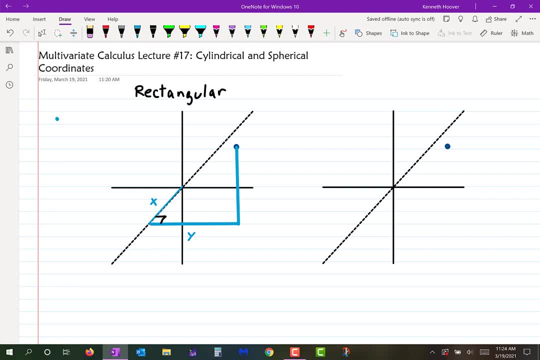 That's parallel to the z-axis And that's our z coordinate, And then that point is labeled as x, y, z. So that's the rectangular coordinate system that you're used to. Okay, now in cylindrical coordinates it's a bit different. 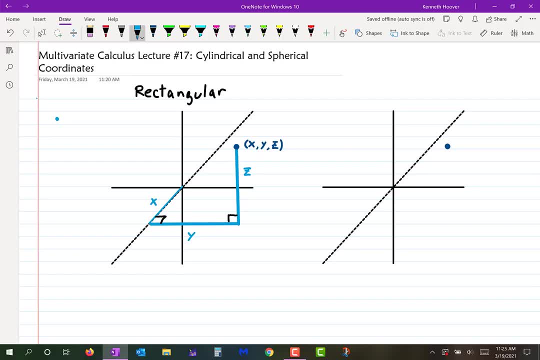 What we do is we go from the origin in the x y plane. We go from the origin straight out to the point directly below our point, Okay. and then we go straight up to the point- Okay. Now this will be perpendicular, right here. 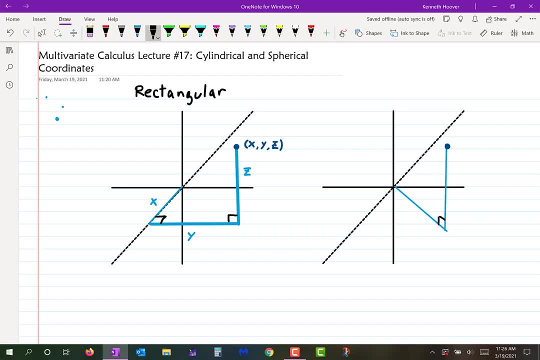 Okay, Now what we do is we measure this angle from the positive x-axis to the blue line that I drew, going straight out from the origin to the location in the x y plane directly below the point. Okay, So we measure that angle and we call that theta. 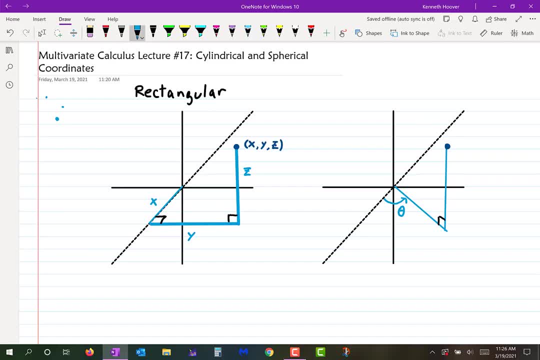 We measure the distance, what is called the radial distance, from the origin to the point on the x- y plane directly below our point, And we call that r, And then the height of the point we call z, And then the point will be labeled with three coordinates. 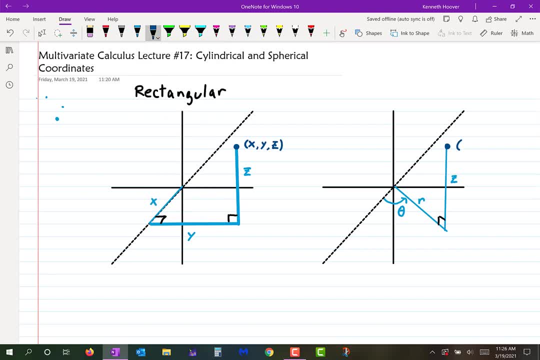 And instead of x, y, z, they are r, theta, z. Okay, that is called cylindrical coordinates. Now you will recognize this right away: That this is simply polar coordinates. that we have already learned, with a third z coordinate added onto it. 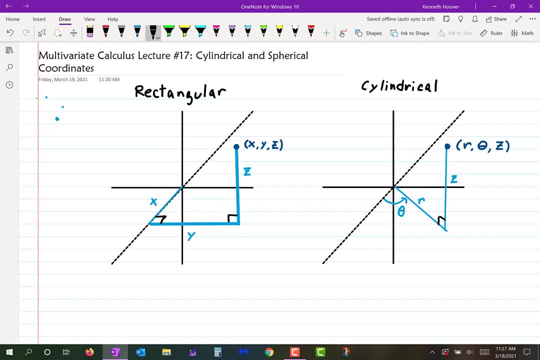 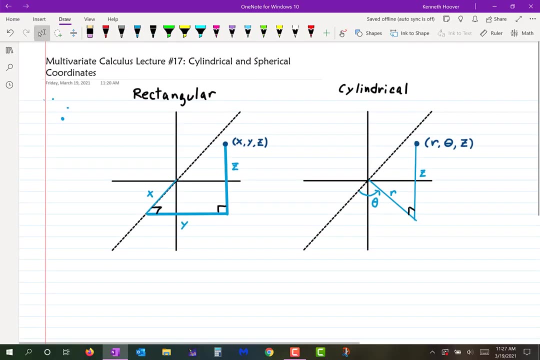 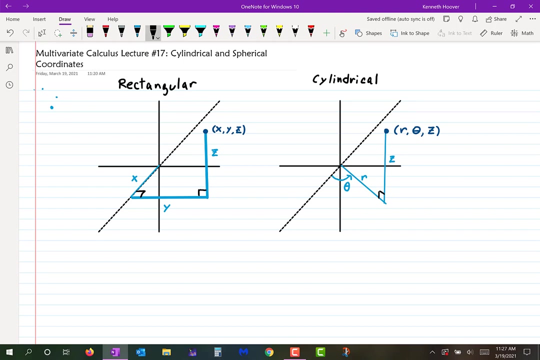 That is all. it is Okay. Horizontally it is polar coordinates And vertically it is rectangular. Okay, So that means that the conversion formulas We already know. Okay, If you want to go from rectangular coordinates To cylindrical coordinates. 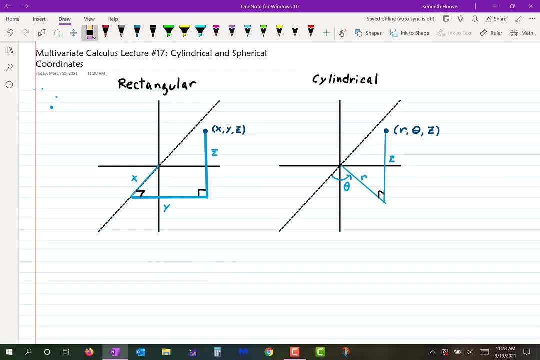 Let me actually move that over. So let's put it this way: If you know the rectangular coordinates of a point- And this works not just for individual points, But also for equations of surfaces as well- If you know the rectangular coordinates And you want to write it in cylindrical coordinates, 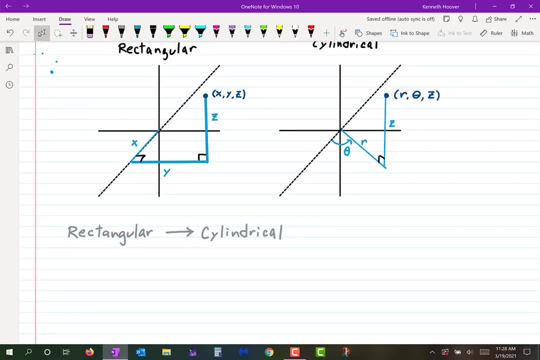 Okay, Then it is really easy. You would know what x, y and z are. You want to find r, theta and z? Okay, Well, r is equal to the square root of x squared plus y squared. Theta is equal to the arc tangent. 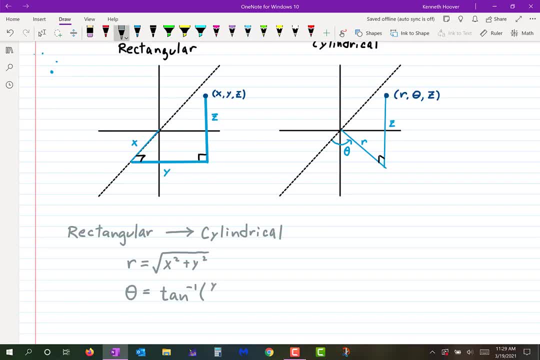 Of y over x And those two are the same equations. we used Several sections back When we were doing polar coordinates. That is all. it is The same. two equations, Okay, And z Equals- z. Okay, If you want to convert from cylindrical coordinates. 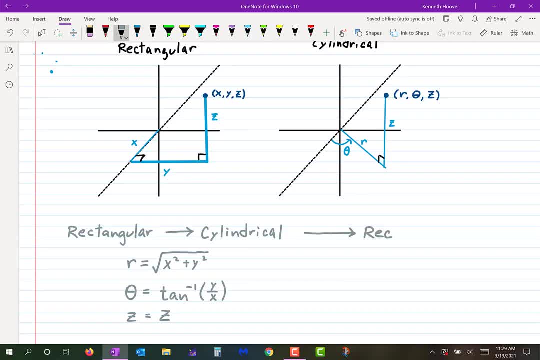 Into rectangular coordinates, Then that means you would know r, theta and z. You want to find x, y and z. Well, again, It is just the same equations that we used in polar coordinates: x equals r, cosine theta. 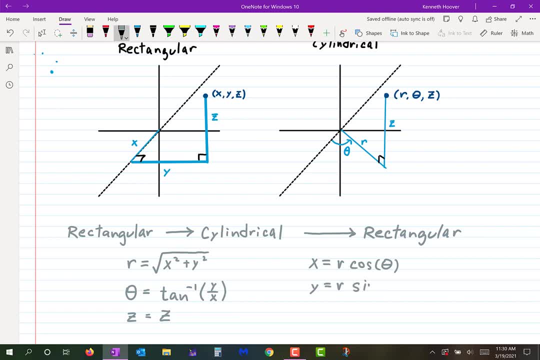 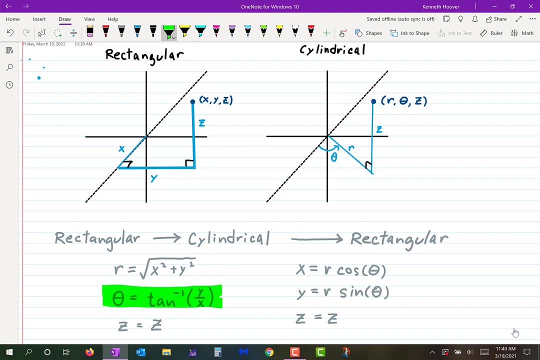 y equals r, sine theta, And z equals z. Okay, Now, this is the way it is presented in most books. However, This part right here is very misleading, And I am going to do it a little bit different way. Here is the problem. 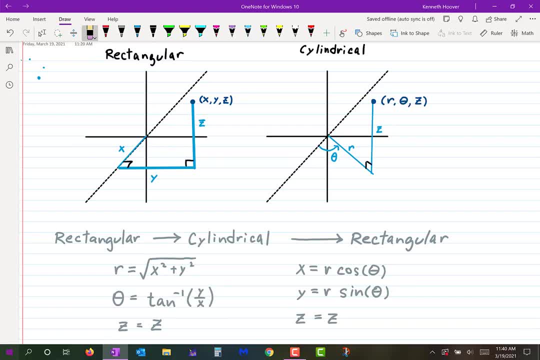 The way things are written right there, r can only be positive, Right Or zero, Because r is the square root of something, So it can't be negative. Okay, And tangent If tangent equals. I am sorry, Not tangent. 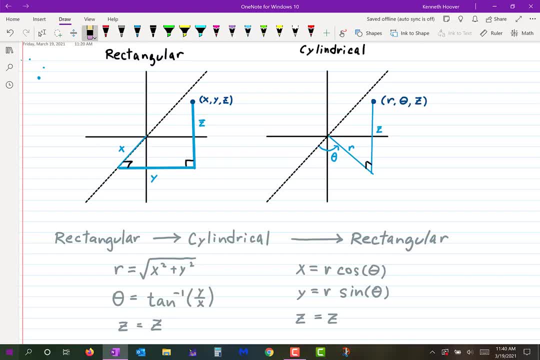 If theta equals the arctangent of something, Then that means theta can only be between negative Pi over two And positive pi over two. Okay, This is a problem And most books kind of ignore this problem. Okay, And think that you will figure it out. 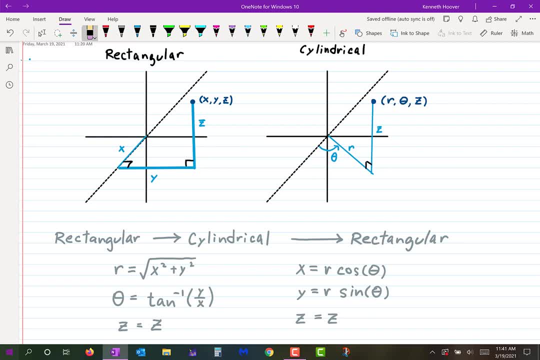 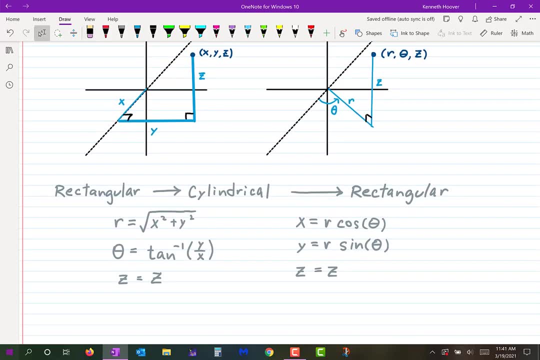 So I am going to write it In a more correct way. That doesn't lead into this problem. Okay, What I am going to do is Number one: Instead of writing, theta equals arctangent of y over x. What I am going to do is I am going to write: 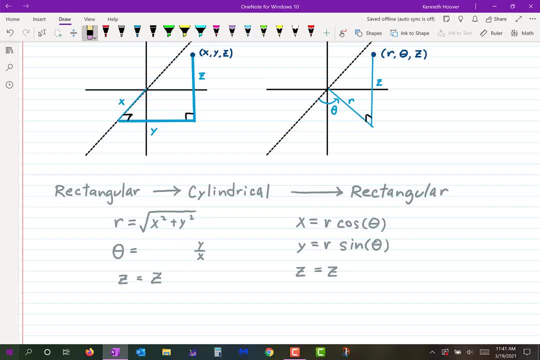 The tangent of theta equals y over x. Okay, Because then I am not using the word arctangent, So I am not limiting myself between negative pi over two And pi over two By saying tangent of theta equals y over x, Then theta can be anything. 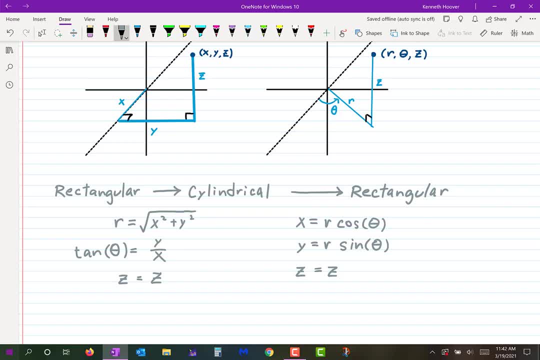 Between zero and two pi. Okay, Now You know that angles in quadrant one Have the same tangents as angles in quadrant three. Angles in quadrant two Have the same tangents as angles in quadrant four. So, for instance, If y is seven and x is seven, 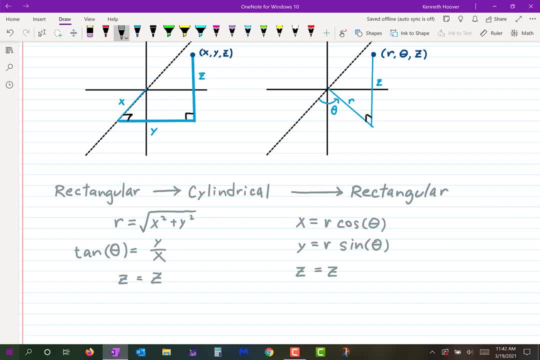 Then y over x would be one. Tangent of theta would be one. Would theta be pi over four, Or would it be five pi over four? Right, So I need to add on here. We will put it right underneath. Let's just get some room here. 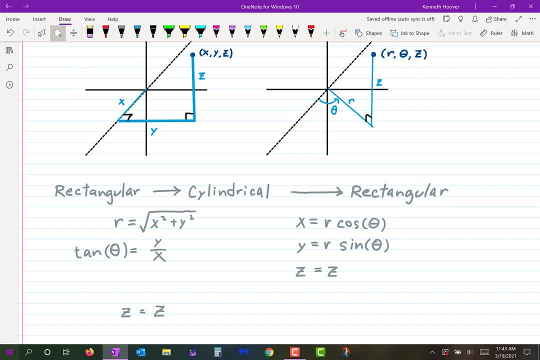 Okay, that Theta Goes from zero To pi If y Is not negative, And theta is between pi And two pi. If y is negative, Then theta is positive seven. Okay, So if y and x are both positive, seven. 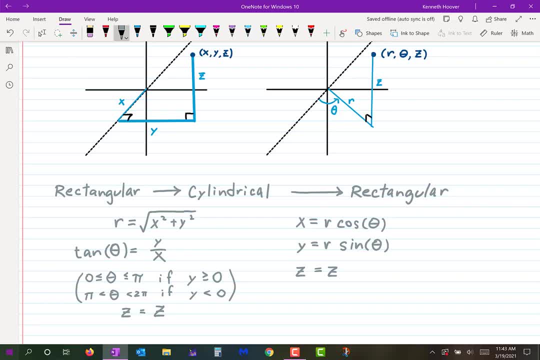 Well, you know that that point then is in quadrant one. The point seven, seven is in quadrant one. So you would say tangent of theta equals seven over seven. So tangent of theta is one. So theta could be pi over four, Or five pi over four. 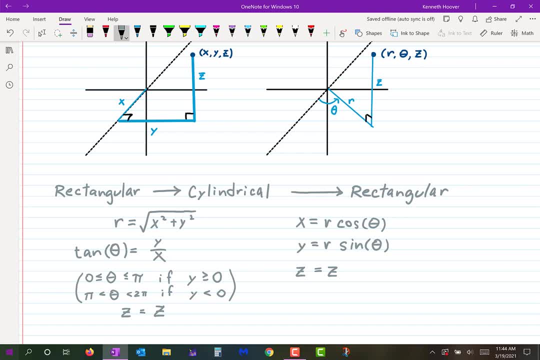 But because seven is positive, Then theta is positive. Then theta would be between zero and pi. So you know it would be pi over four And not five. pi over four If you had, X and y are both negative three. So that's the point. 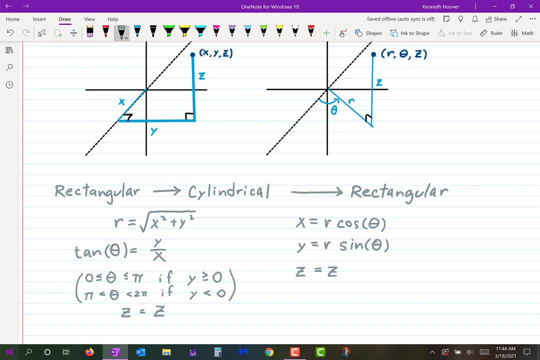 Negative three, negative three. You know that's in quadrant Three. So you would have: tangent of theta equals negative three over three, Which is one. So tangent of theta is one. So theta might be pi over four Or five, pi over four. 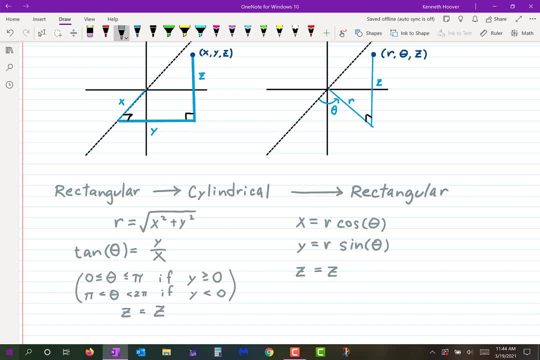 Because negative three is a negative number. Theta would be between pi and two pi, So it's not pi over four, It's five pi over four. Okay, Now let's do some practice Here. I'm going to write down this equation here: 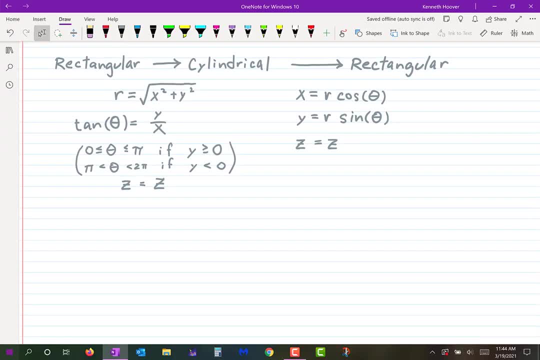 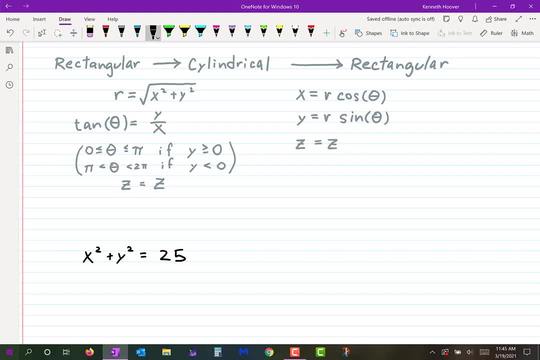 Into Cylindrical coordinates. Okay, Let's convert that equation into cylindrical coordinates. So Let's think about r: R equals the square root of x squared plus y squared, So that's the square root of twenty five, So that's five. 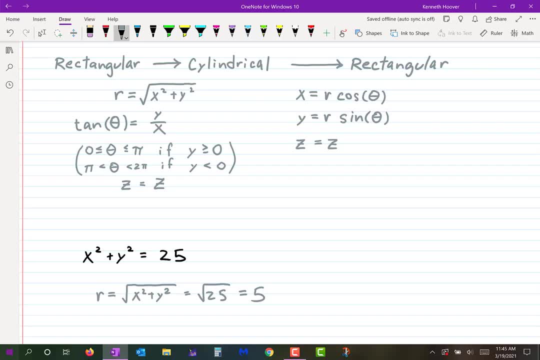 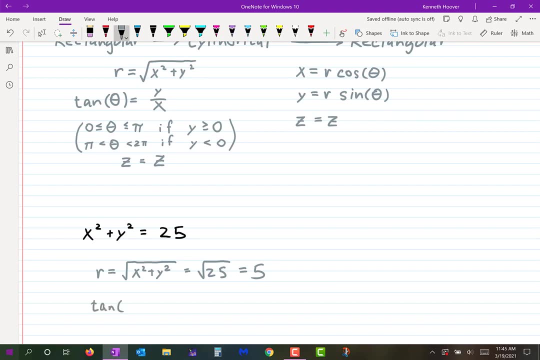 Okay, R must be five. Now let's think about theta. The tangent of theta Has to equal x. I mean y over x. Now I know any restrictions on what y over x must be. I know that x squared plus y squared has to equal twenty five. 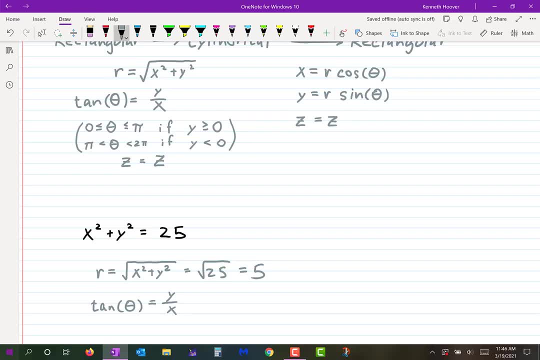 So there's a definite relationship between x and y. That puts a restriction on x squared plus y squared. It also puts a restriction on x And a restriction on y. We know that x and y individually Range from negative five to five. 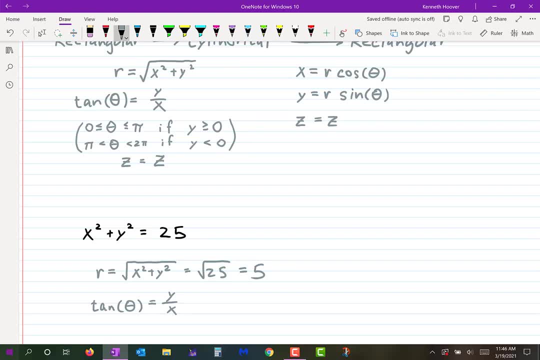 They can't be outside of that range If the sum of their squares is twenty five. But I claim that I don't know anything at all about X over y. X over y can be anything from negative infinity to infinity. Okay. 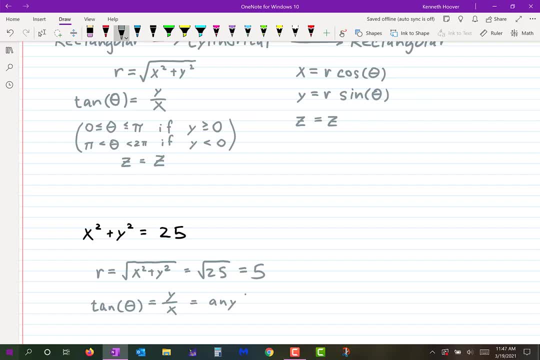 I'm going to write that down. I'll explain why. I know that. For instance, What if y is five? X can be anything from negative five to five. So let x go to zero, Then y over x will go to infinity. 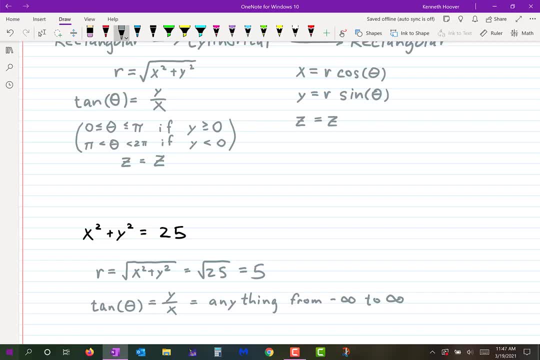 What if x is? What if y is negative five And x goes to zero From the left, Or sorry, rather from the right, Then y over x will go to negative infinity. So y over x can be anything From negative infinity to infinity. 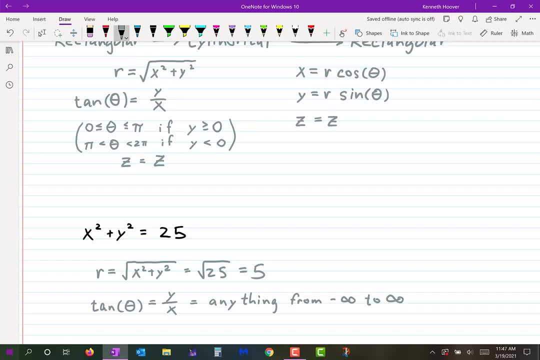 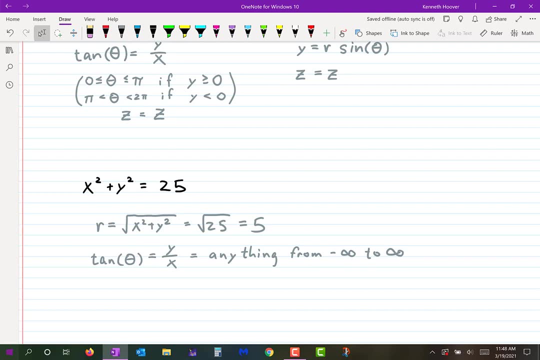 So tangent of theta can be anything from negative infinity to infinity, And so that means theta Can be anything Between zero and two pi. Okay, And now let's think about z. Is there anything in the equation that's putting any restriction at all? 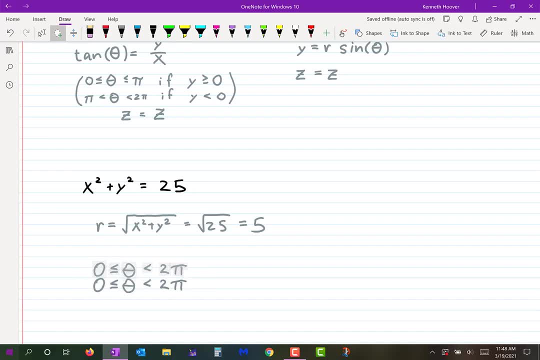 On z: No, z is not even mentioned in the equation, right? Does that mean that z doesn't exist? No, It just means that z could be anything. Okay, So r must be five. Ends up being the only restriction that I have. 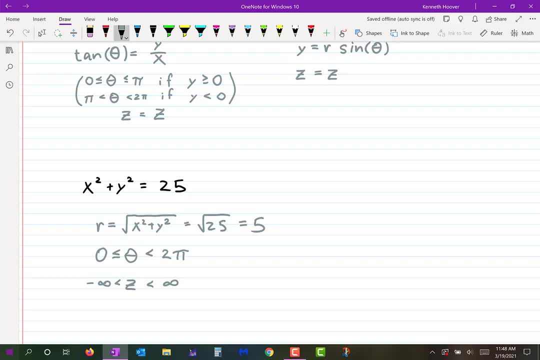 Theta can be anything, Z can be anything, Okay. When I say theta can be anything, I mean any angle. But we always, We restrict ourselves between zero and two pi, Right, Okay. So that means the equation X squared plus y squared equals twenty five. 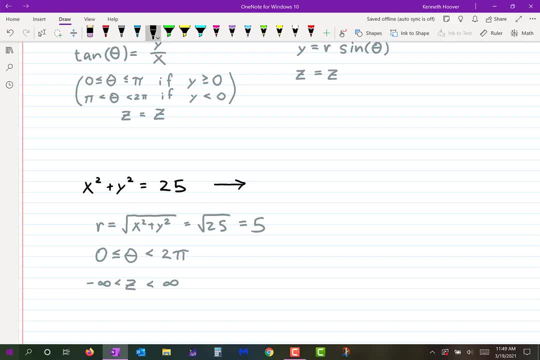 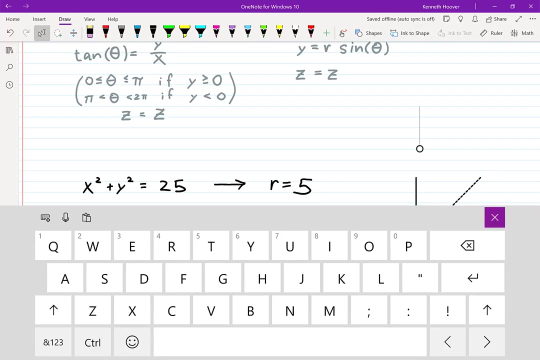 That's a rectangular equation. When I turn it into a cylindrical equation, It just becomes: R equals five, Theta can be any angle, Z can be any number. So what would that look like if you tried to graph it? So I want you to think about this for a minute. 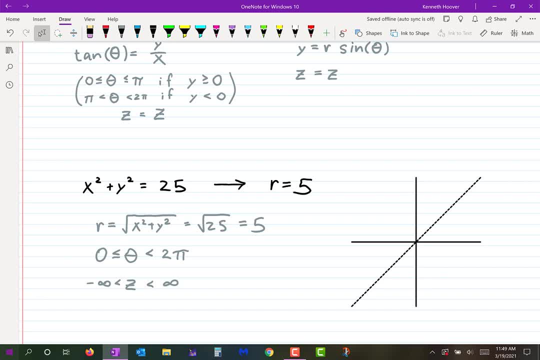 Okay, R equals five, So every point is five units away from the origin, Or actually, what I shouldn't say the origin here, I'm sorry. I should say from the z axis. Every point is five units away from the z axis. 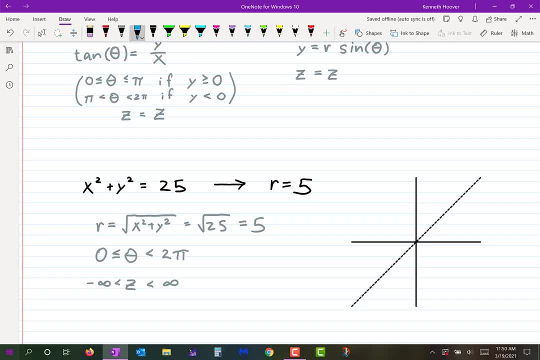 But theta can be anything. So, let's, let's do this, Let's draw this line here: Okay, Five units away. Okay, But theta can be anything. Okay, Theta can be anything. Let me draw that so that it looks like it's flat on the x- y. 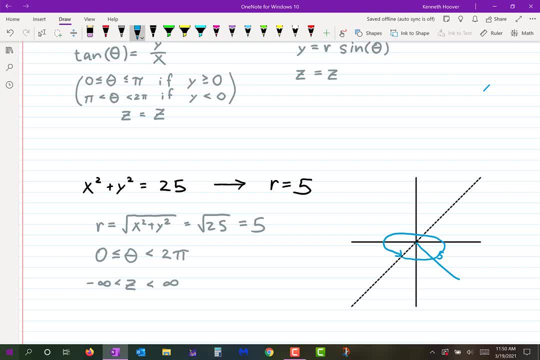 Okay, Theta can be anything, So that that line that I drew, that's five units long, can swing around in any angle. And what would it do? Oh, it would work without a circle, wouldn't it? Oh, yeah, Okay, Okay. 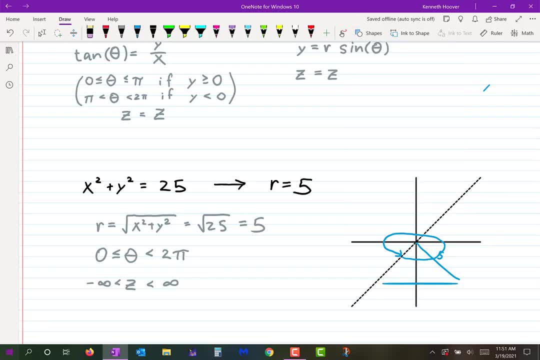 Yeah, Okay, Okay, Yeah, Yeah, Okay, Yeah, Okay, Yeah, Yeah, Okay, Okay, Yeah, Okay, Okay, Okay, Okay. Sorry, I'm trying to Darn it. Okay, Okay Yeah. 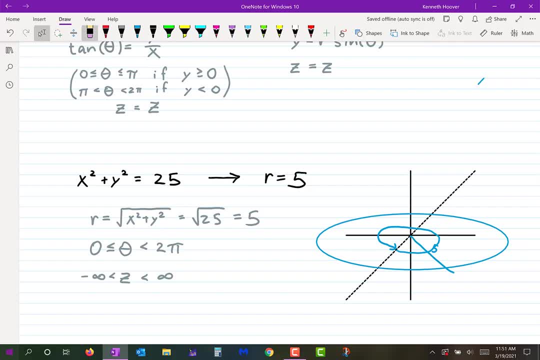 Okay, Okay. well, that's good enough. Okay, now what else? Z can be anything, So that circle can move up and down. What do you think we're going to end up with? We're going to end up with a perfect cylinder. 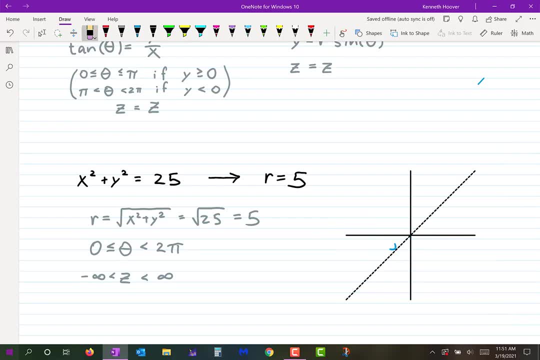 Okay, let me try to draw it here for you a little bit better. Okay, that's what the equation would look like. That's a cylinder. I drew it like it has a top and a bottom so you could see the shape, but it would actually. 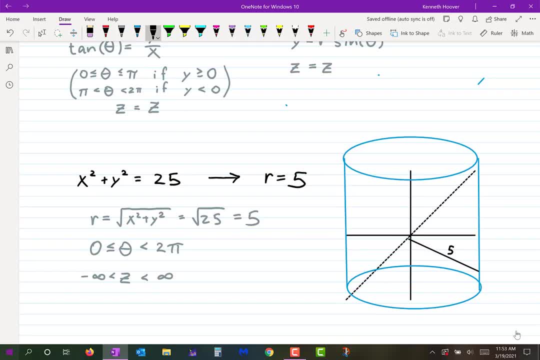 go up forever and down forever. It doesn't end at the top or the bottom. Okay, that's the equation. r equals 5. Every point on that cylinder is 5 units away from the center of the cylinder, But it can't have any z coordinate and any theta coordinate. 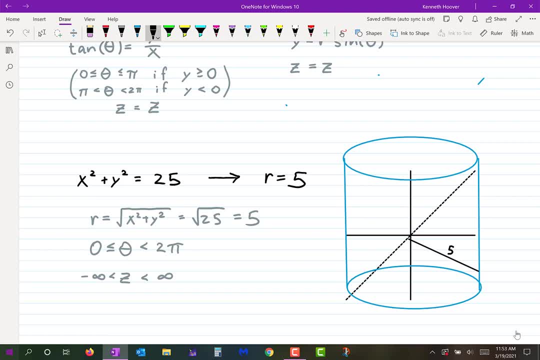 Okay, It takes a little bit of getting used to with the graphs. Doing the math of converting is easy, but getting your mind around the graphs is a little bit trickier. It's going to take some practice. Okay, All right. now there's something called spherical coordinates. 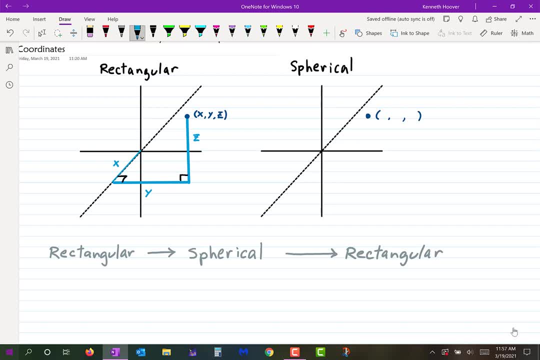 Okay for spherical coordinates. what we do is, instead of measuring an x and a y and a z, like I have in the picture there of rectangular coordinates, what we do is we draw a line segment from the origin straight out to the point wherever the point is floating in space. 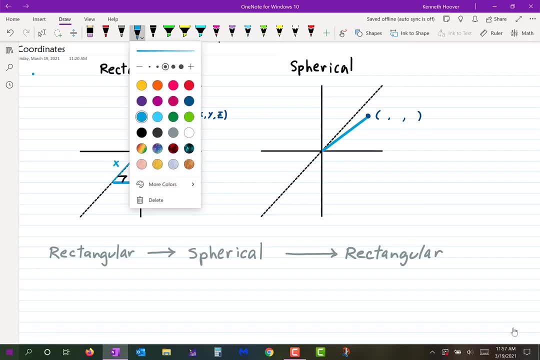 Okay, So here's one. Okay, So this is 90 and that's 0.. We're going to call row: That's 45, right there, So that's 45 and that's on the x axis. So then you divide 45 by 2, find where the point is. 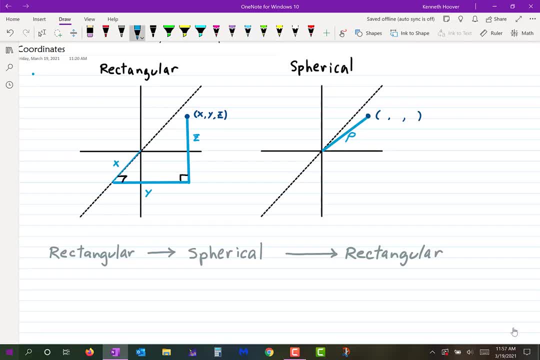 Now the other thing that we do is we measure the angle from the positive z axis down to that line, segment 7.5 there, and then that's 22.5.. We call that angle. We call that angle phi. I like to draw my phi's like that. 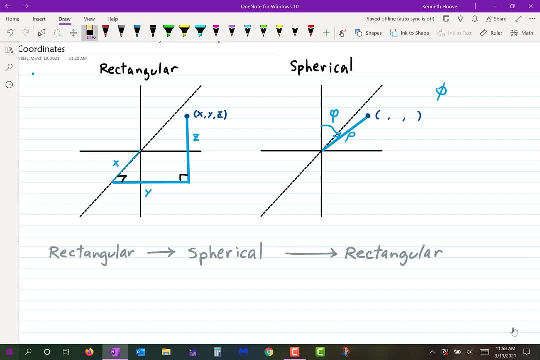 In books they often look like that. Okay, but I don't like that so much. Okay, And then one other thing we do is we look at the shadow of that line segment on the xy plane. Okay, so I go straight down. 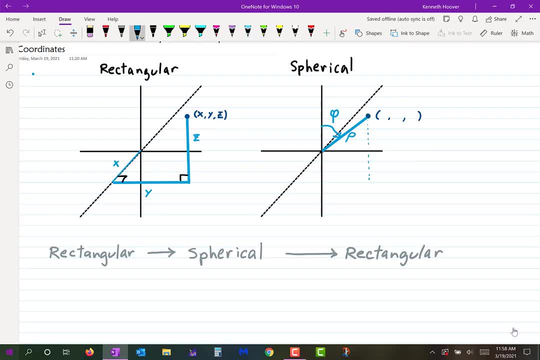 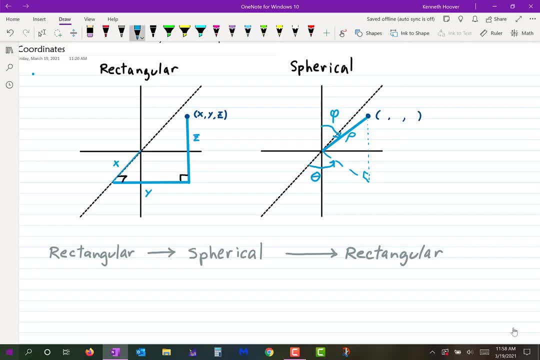 Just like it is. Theta is just like it is in cylindrical coordinates. okay, And so Our point will be labeled with, instead of an xyz coordinate, our point will be labeled with row, which tells us the length of the line segment from the origin to the point. 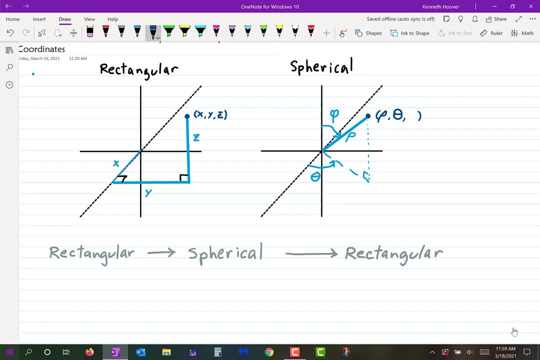 Theta, which tells us the angle in the xy plane from the positive x axis to the shadow. Theta, which tells us the angle in the xy plane from the positive x axis to the line segment, And phi- some people say phi- which tells us the angle from the positive z axis to the 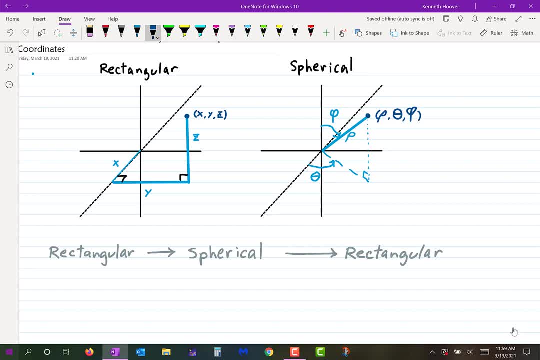 line segment. Oh my gosh. Okay, that's called spherical coordinates. Now how do you convert from one to the other? Alright, Yeah, you're right If you know the rectangular coordinates. so you know x, y and z, and you would like. 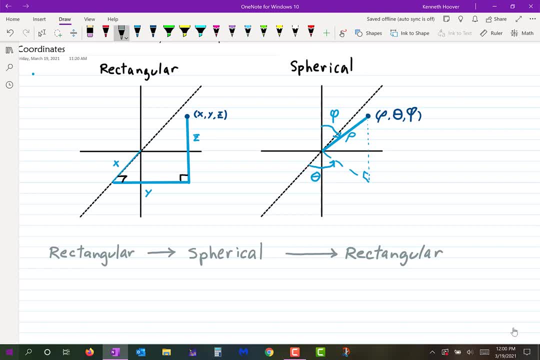 to find the spherical coordinates. you use these equations And row: equals the square root of x squared plus y squared plus c squared. Theta is just like it was for cylindrical coordinates. so I'm going to write: tangent of theta equals y over x. 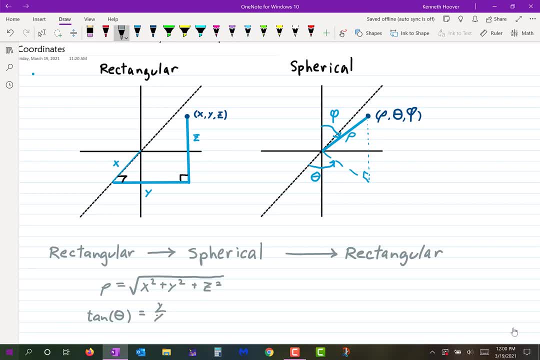 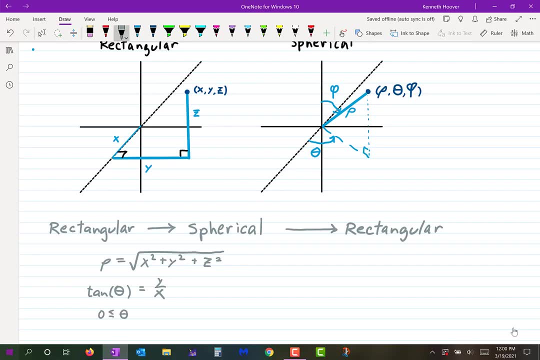 Okay, Yeah, Okay, Okay, Okay. And I'm going to add there that theta is in quadrants one or two if y is not negative, and theta is in quadrants three or four if y is negative. No, I think I'd go back and read both of them. 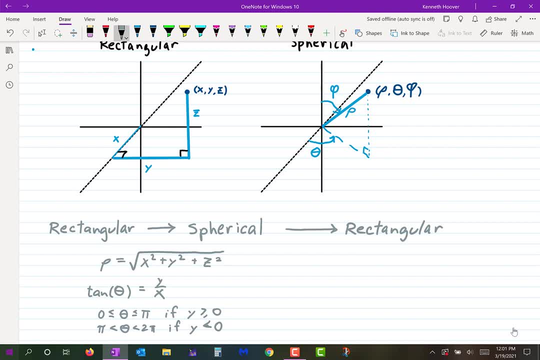 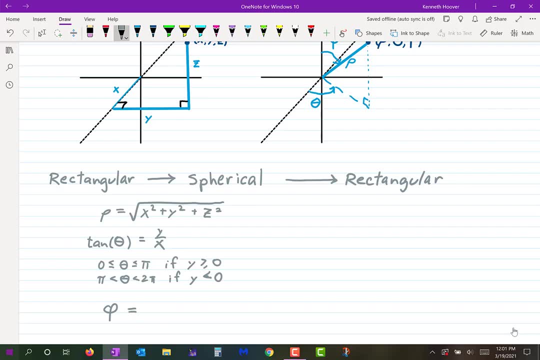 Okay, I'll go a lot more. Okay, Okay, Okay, Yeah, Okay, Yeah, Okay. Here's the second one. So here's the third one. Oh, okay, Okay, Okay, And we're going to find phi. 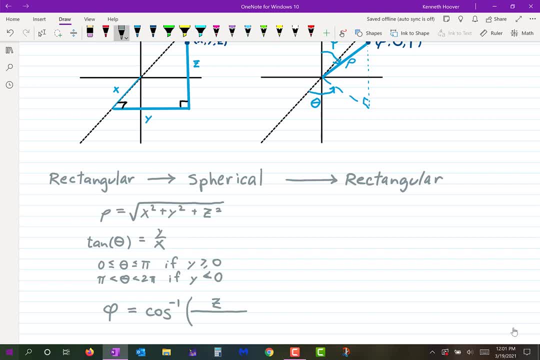 Okay, Okay, Okay, Yeah, that's right. That's right. Phi or phi equals the arc cosine of z divided by row. Okay, Great, Thank you for joining us, And I'm going to stop here, and we are really looking forward to the next question. 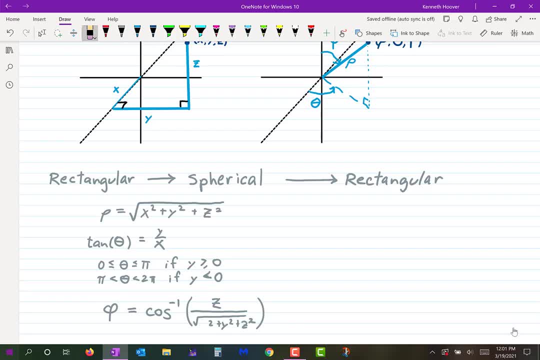 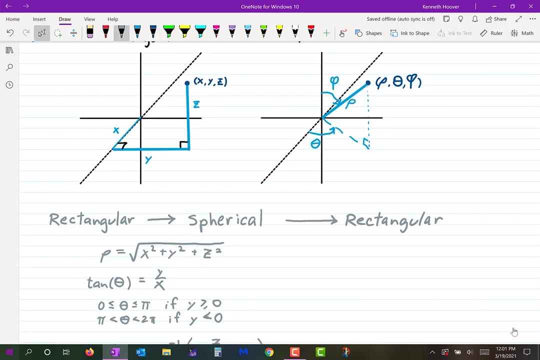 Okay, Bye, Thank you, Bye, Bye, Bye, Bye. Oops, I'm sorry, I almost drew a Z where I should have drawn X. Okay, If you look at the picture, that would make sense. I don't want to make the picture too crowded here, but if you just look at that right triangle, 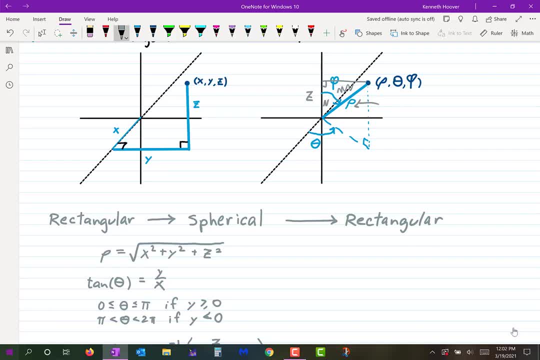 right here, Here's Z, here's rho, and this angle phi would be the cosine of phi would be adjacent over hypotenuse, so that would be Z over rho. So phi is the arc cosine of Z over rho. That's why that's the case. 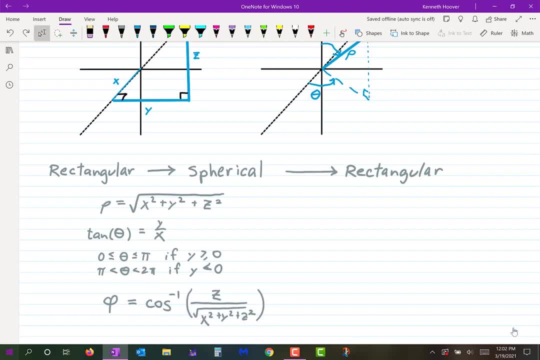 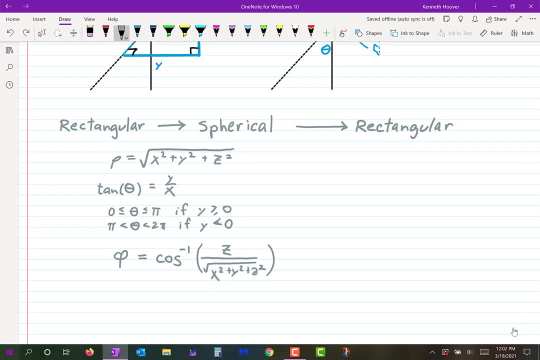 Okay, Now, if you know the spherical coordinates of a point And you would like to write the rectangular coordinates, then here's the conversion equations: X equals phi- I'm sorry, rho sine of phi, cosine theta. Y equals rho sine of phi, sine of theta. 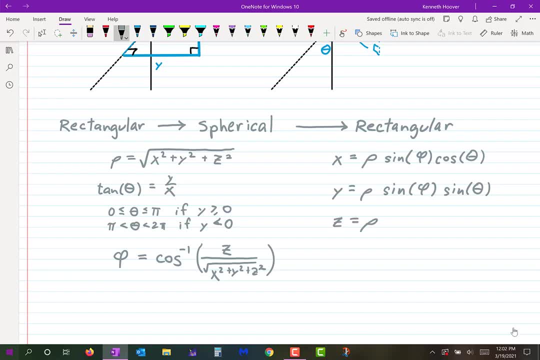 Okay, And Z equals rho, cosine of phi. Okay, So this is how you convert from rectangular to spherical. This is how you convert from spherical to rectangular. Okay. Now, as far as There's going to be some questions, Okay. 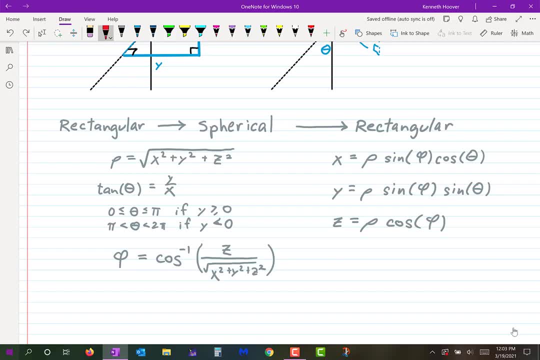 There's going to be some questions in the homework where they give you an equation and they say: you know what would the graph of this look like? You know, that really just takes some practice. It's Yeah, that's right, Captain. 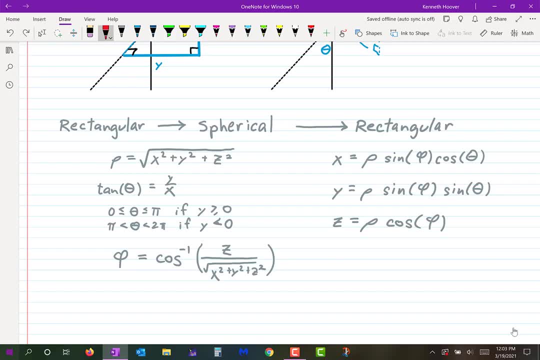 It's very difficult. In fact, I don't even know is it really possible to prepare you for that other than to just have you do some problems and you'll gain some intuition for it as you go. Okay, I know that might seem to you an insufficient explanation, but you're going to have to look. 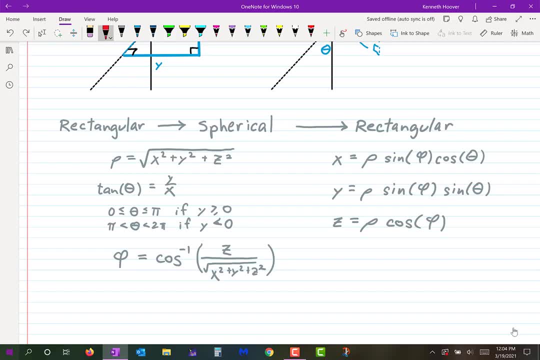 at the problems and look at the choices and just think about you know if the choices they give you- because there are going to be multiple choice- okay, and just think about, um, which one you think it is Okay, Okay. 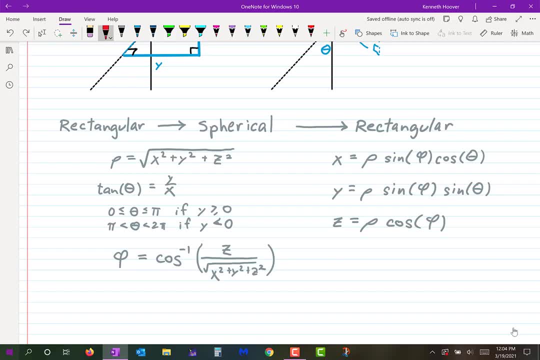 Try that answer and then read their explanation. Okay, Newton is very good about giving explanations, So read their explanation and what will happen is you'll gain an intuition for it. Okay, And other than that, you can also come to my Zoom office hours and ask me for help, and 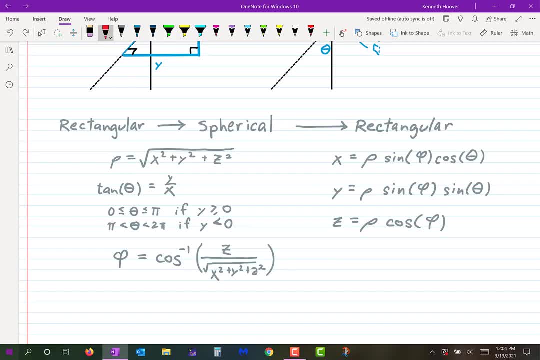 I'll help you with it. Okay, Yeah, All right, That's all for today.